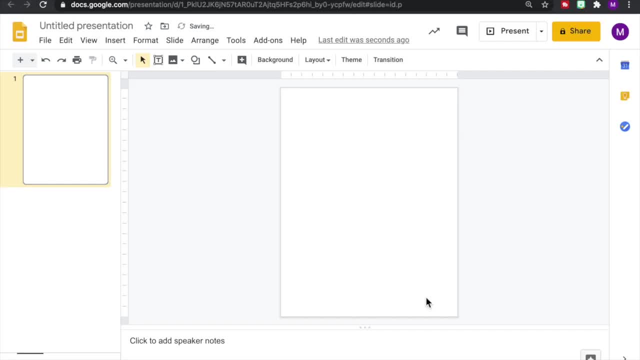 11. 11 inches Hit apply. And there is our page. So we're going to start with the first worksheet. We're going to insert a text box to set up our name and our heading And then we're going to add in our shapes. So let's go to our shapes button in our toolbar And the 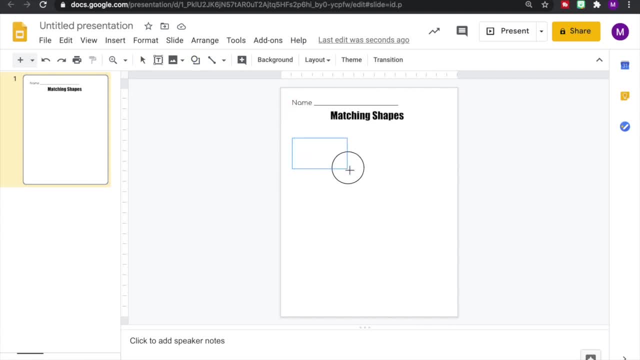 first shape I'm going to use is a rectangle, just going to stretch that out. And then the next shape I'm going to insert is a circle in a rectangle that we're going to shape as a square. we'll add in a triangle and 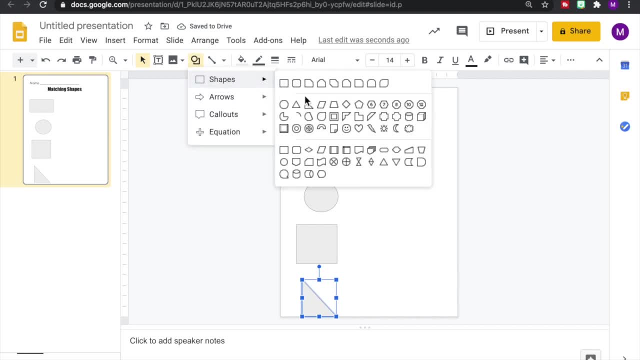 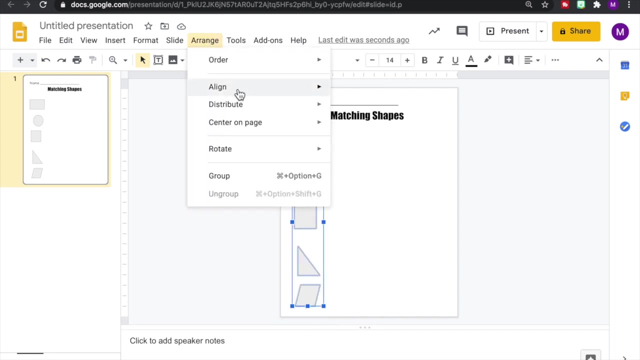 then we're going to add in a rhombus as well, so I'm going to select all of them and decrease the size of the shape. so now they're a little scattered, so what I'm going to do is select all of them, then go to the menu, hit, arrange, hit. 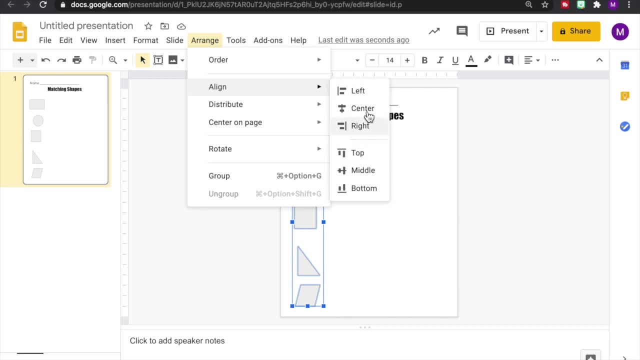 align, hit Center, so they're all aligned in the center, and then go back to a range, go to distribute and then hit align. distribute vertically to make sure that they have the same amount of space in between each shape. then we're going to color in each of our shapes. so let's. 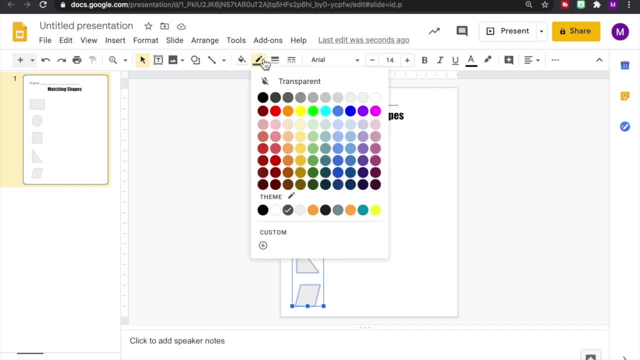 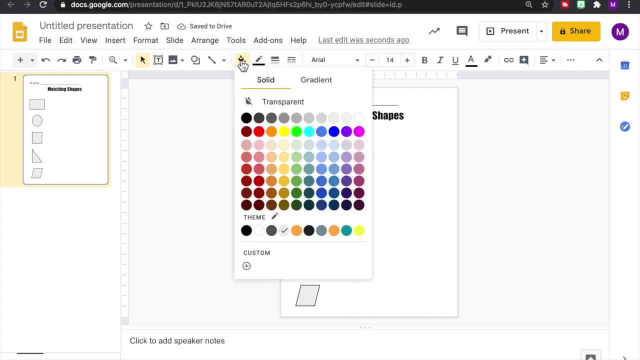 highlight them again. I'm going to click on the border- black border- and then increase the weight of the border and then just give each shape its own color. so there are shapes, so we're going to select the shapes and I'm going to duplicate them. so, using my keyboard, I'm going to 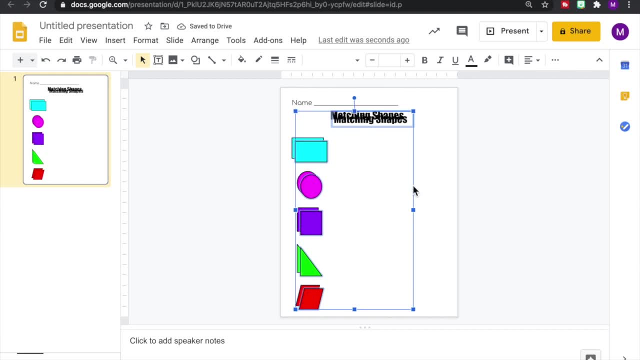 hit command D. you have a Mac. if you have a PC, hit ctrl D. let's move them over. let's get rid of that title. it's going to select those text boxes and then move them in just slightly. let's move these in as well. okay, so now what we want to do is rearrange our 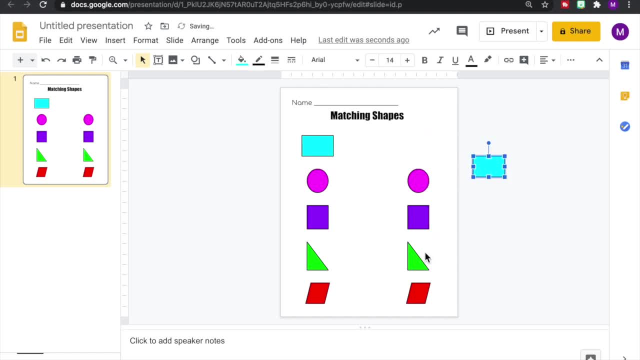 shapes on the right so that the students have to match them. so we don't want them to be in the same order and I'm just going to select them again and make sure that they are aligned. so do, align Center again, arrange and distribute vertically again, and the last thing I want to do is add in a border. so I'm going to go to 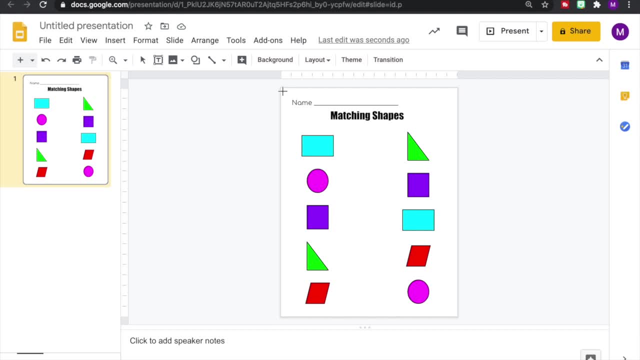 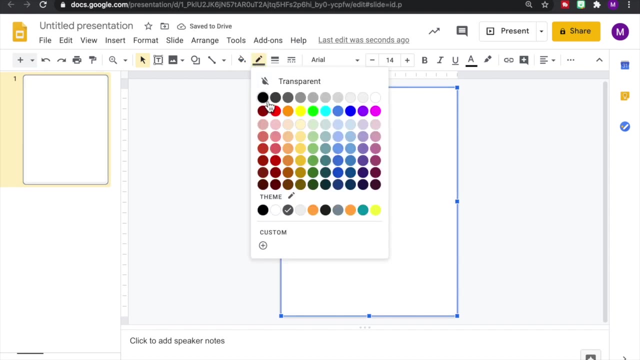 shapes, add in a rectangle and cover the entire page. for the fill color, I'm going to choose white and then the border color: I'm going to choose black and give it a thickness and then right-click with order send to back. so we have our border now. i'm going 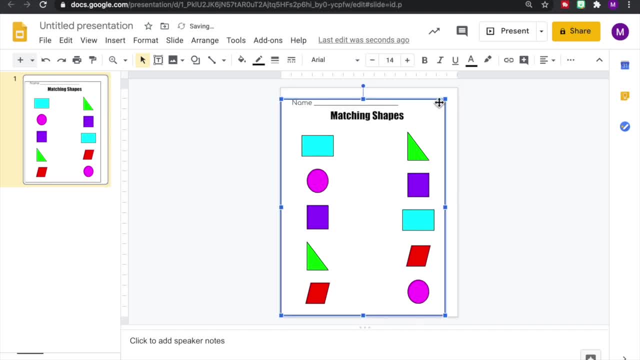 to bring that border in and then just Center it. so there's our first page. let's add in directions really fast, and then we'll be done with this first page, okay, ok, yes, dead directions are added in. so we're done with that first page. now we're gonna. 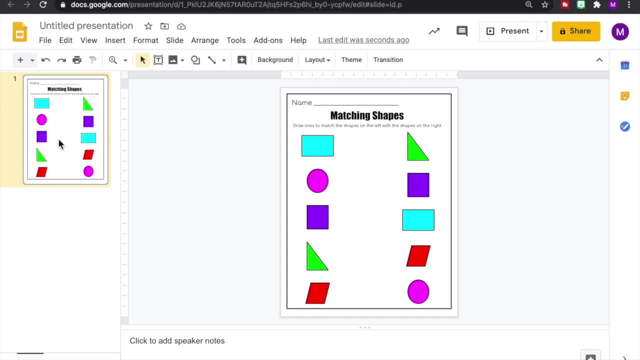 start on our second page. so where our slide is on the right, I'm going to right-click and hit duplicate slide. and now we're working on our second page. so I'm gonna move, I'm gonna delete the border for now. we'll bring it back at. 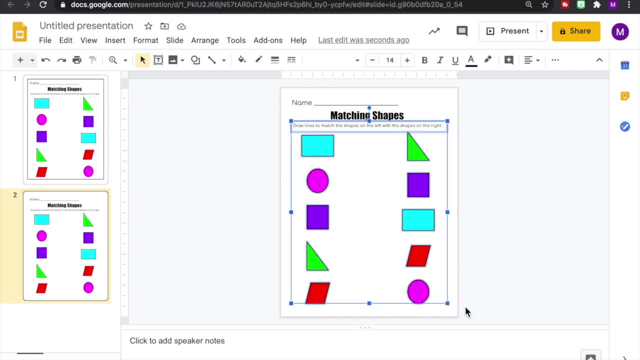 the end, and then we're going to select all of the page or all of the images below, and I'm going to delete those. for this second page, we are going to have students matching numbers and amounts together, so we're going to change that title. this time we're going to insert images from the internet, so we're going. 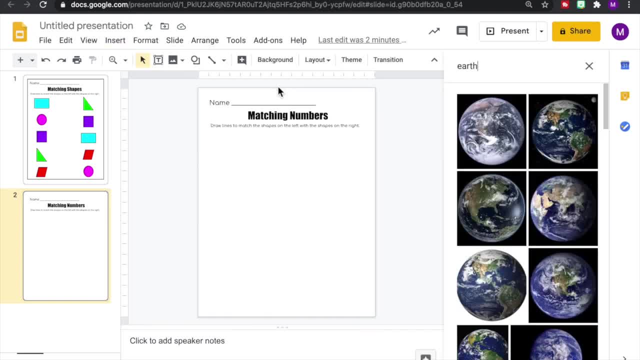 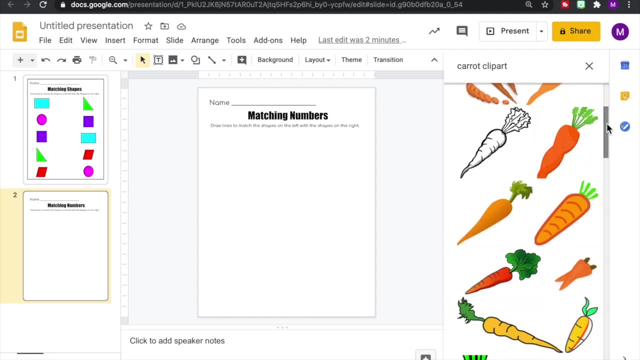 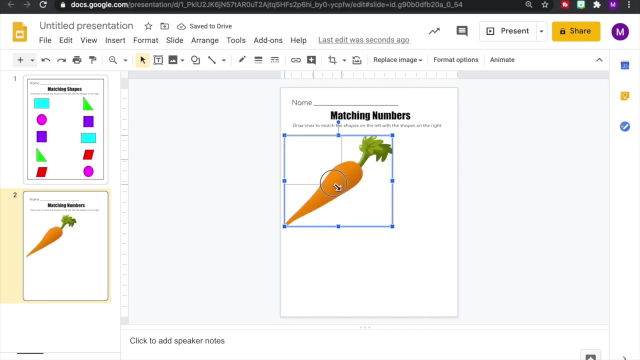 to go to insert image and then search the web. I'm going to type in carrots clip art. so have like a food theme, vegetable theme maybe. I'm going to select this carrot and then click on insert. I definitely want to make it smaller and then I want to change the position of the carrot, make it kind of. 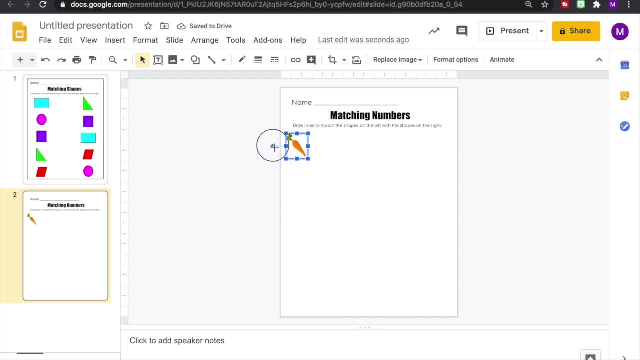 leaning up, and then I'm going to duplicate them. so here you can choose the amount of carrots that you want. so I want carrots, so I'm going to duplicate those carrots. then I'm going to, I'm going to be arranging the carrots, so I'm going to select the first one and the last one to. 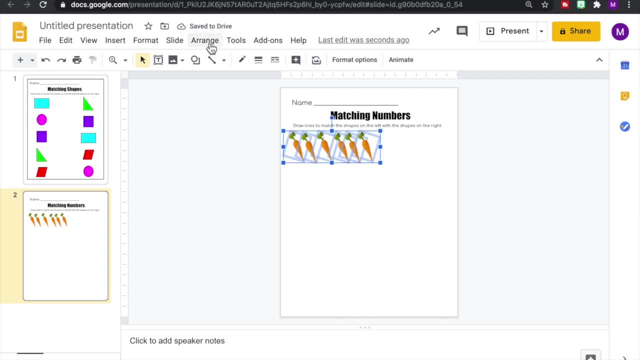 make sure they're lined up. and then I'm going to select all of them, go to arrange a line, align middle, arrange, distribute, distribute horizontally to make them, make sure they're aligned. and then I'm going to select them, right click and go to group so they're grouped together, and then 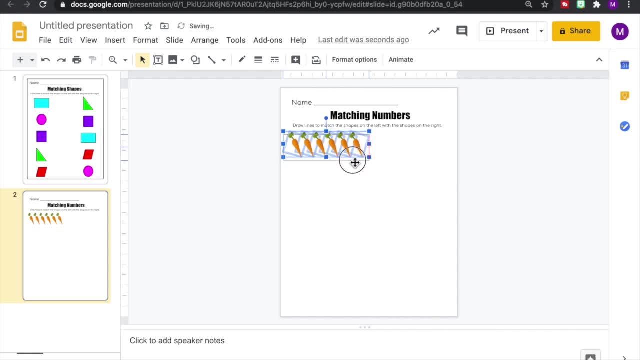 I'll probably decrease the size just slightly one more time. so there's our carrots. let's do another image. we're going to do corn this time, so insert image. search the web type in corn clipart. this one looks good: insert. so let's change the direction and then minimize. 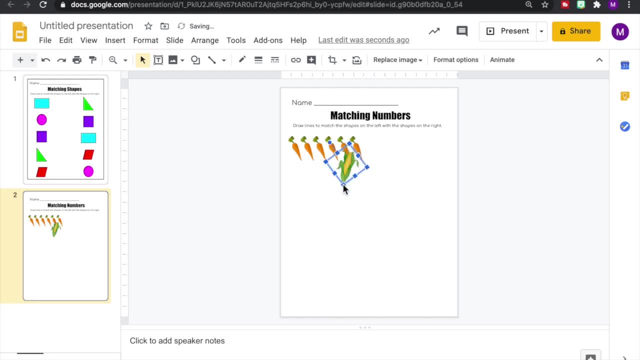 that corn. remember, this is just to give you ideas to inspire thinking when it comes to creating activities and printables for your students. so definitely use what you want. make it what you want it to look like for your children and your students. let's make it a little bit smaller. so I want four corn, so I'm going. 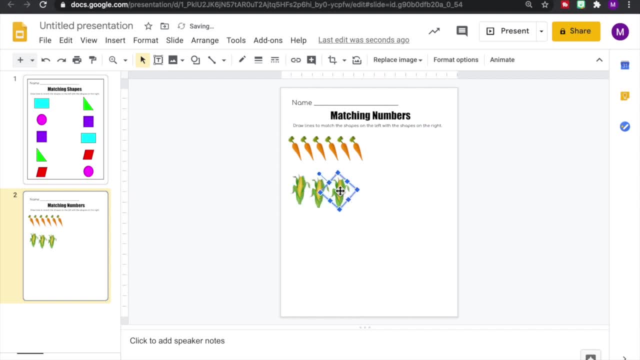 to duplicate the corn, and then I'm going to line that last one up with the carrots, where the carrots end, and then let's arrange them so that we have five sets of numbers and then we'll add in our numerals. those are done. let's select, right click and group them together. I'm going to add: 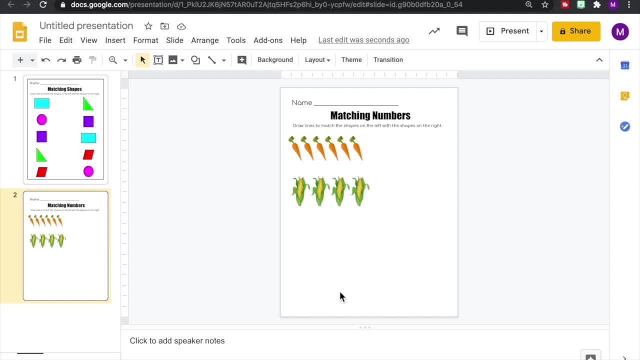 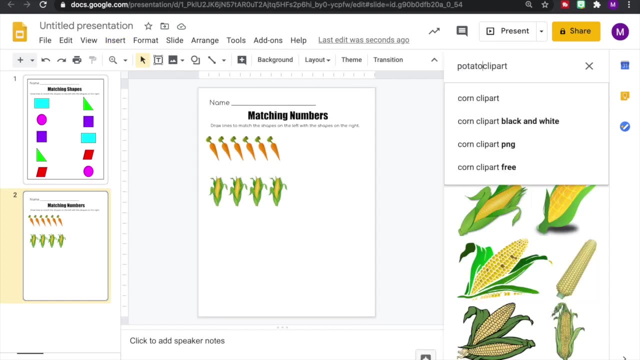 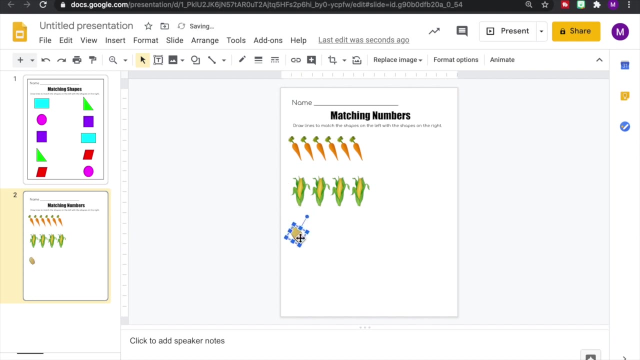 in three other vegetables to our page, so that we have five sets of numbers, and then we'll add in our numerals. so that's one bite size, four inside out. so there we go, this huge, unnecessary thing. seven, four V's, that little five, and then I'm going to go ahead and insert. 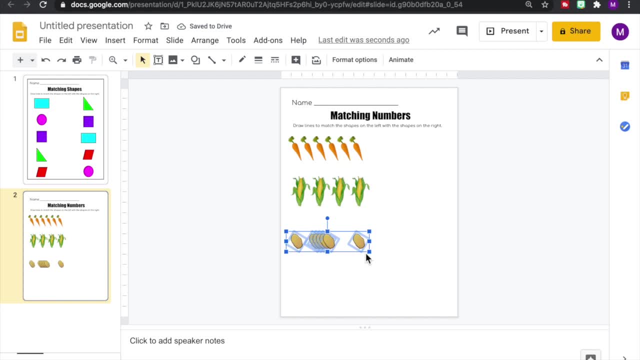 it inside out first guess I'm going to use this caregivers miles size and this is a insert one in here so we can get at from three, two, three and one begins selecting on one of these ready to share. the viewers are going to want these here together first, and then I'm going to select the last and I'm going to enter all of the. 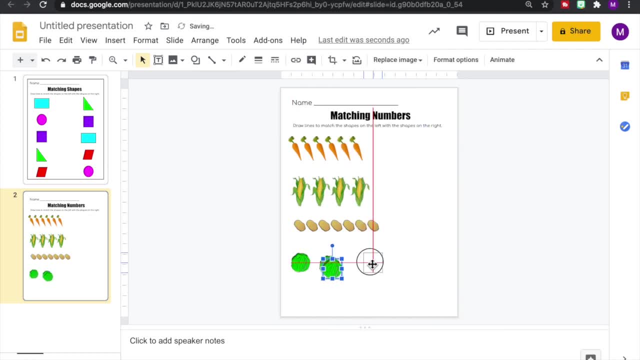 Thank you. Okay, so we have our pictures of our vegetables and our number amounts ready. Now we're going to add in our numerals. So I'm just going to add a text box and type in a number. So let's start with seven. 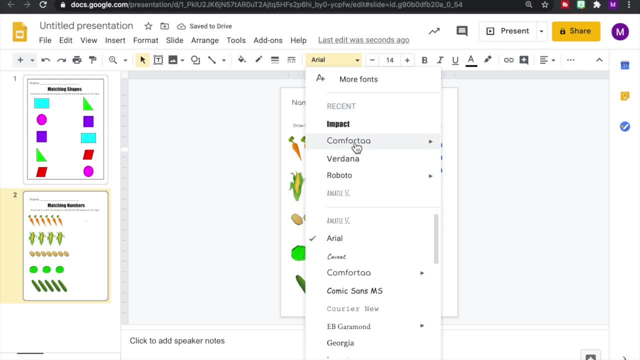 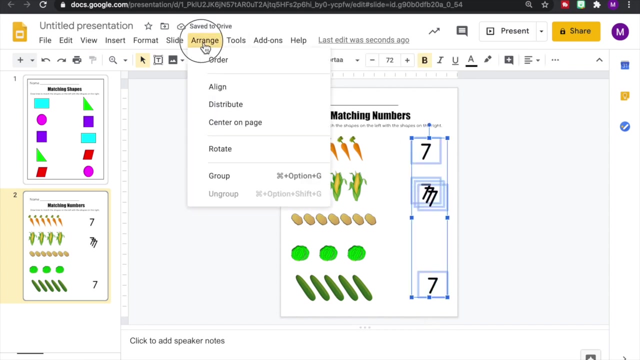 Let's change the font and then increase the size, Let's center it, Then I'm just going to duplicate that text box, Okay, And then bring that final one down here, And then let's select them all and arrange, And then we're going to adjust our numbers. 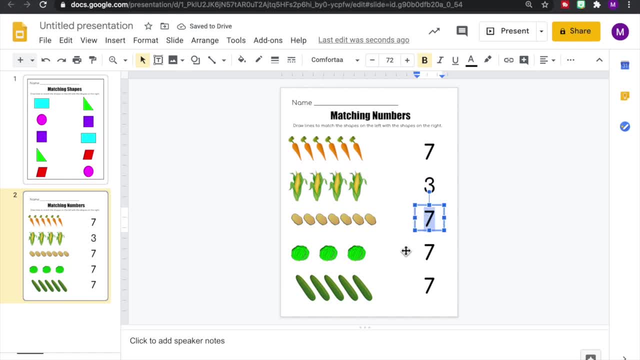